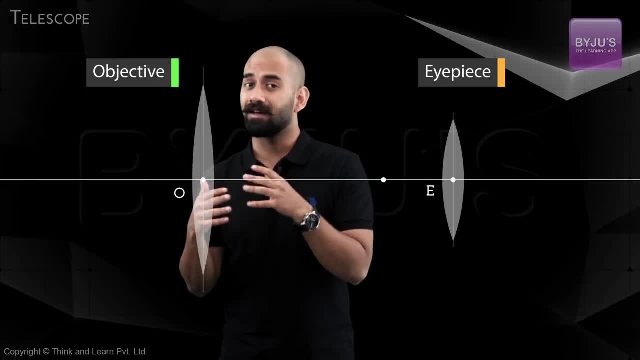 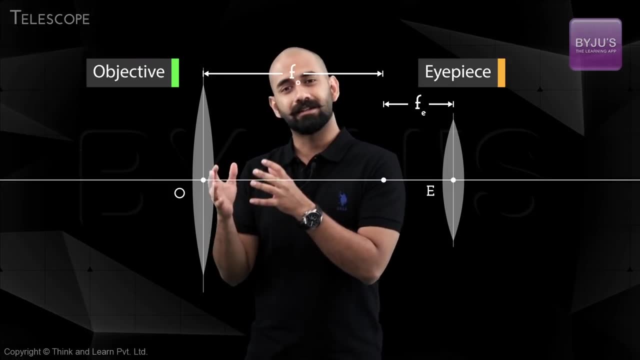 Now, the only difference here is that the objective has a larger focal length and the eyepiece has a smaller focal length. We will come to why in some time. So what happens is so: the objective receives parallel rays because the object is extremely far off. So 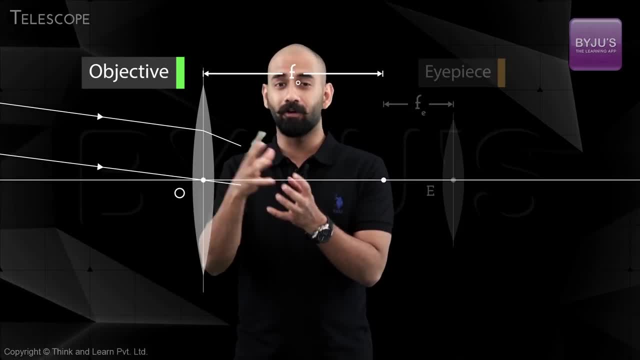 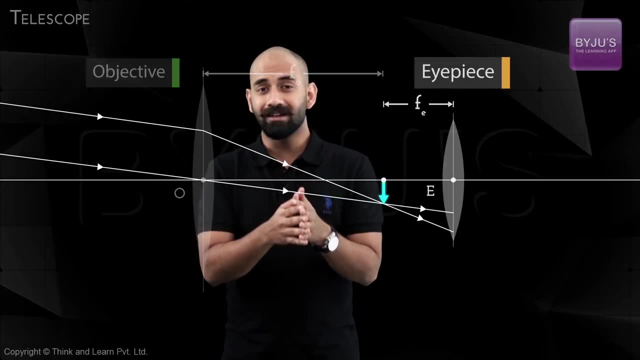 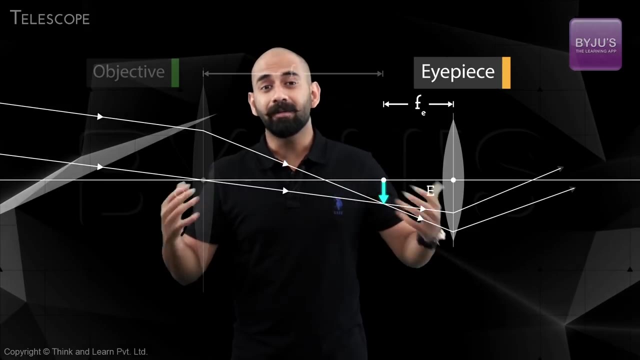 it is almost at infinity. So these parallel rays are focused by the objective and it forms a real inverted and diminished image. Now the thing is, the eyepiece is placed in such a way that the image is formed at the focus of the eyepiece itself. So therefore, the 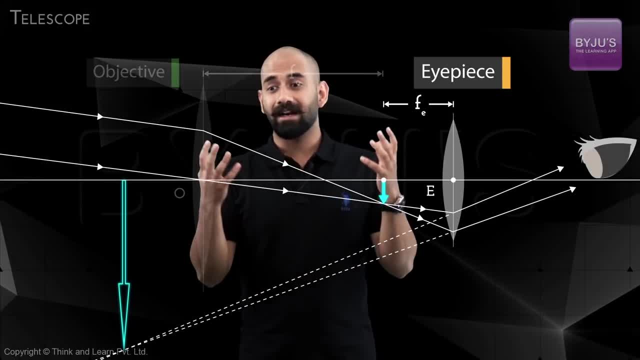 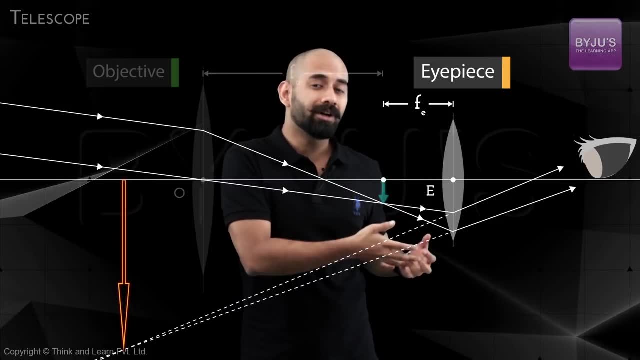 eyepiece forms a virtual, inverted and magnified image of this particular image. Why? because this image acts as an object for the eyepiece. And why is the image inverted? Because this image also is inverted. So, as I said, you finally end up having a 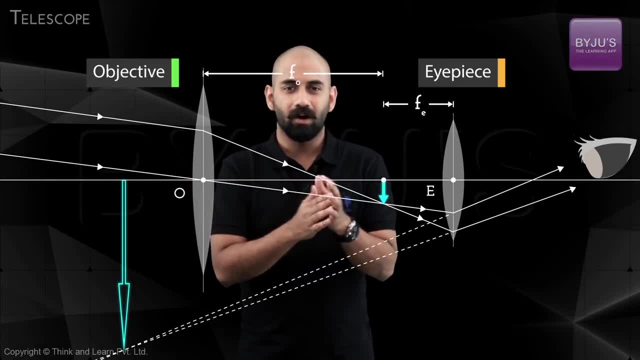 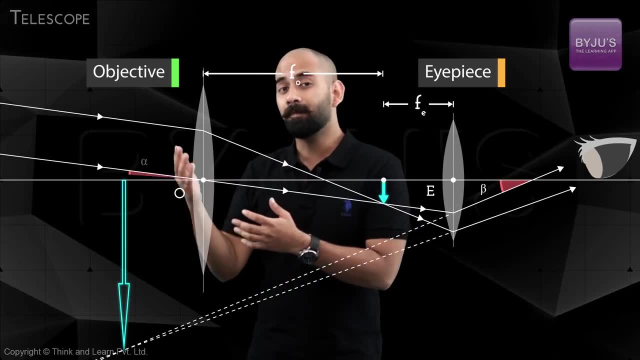 virtual inverted and magnified image. Now, if you see, you can see that the angle subtended by this image at the eye is greater than the angle that the object was drawn at. When you object subtended at the eye. so therefore, this is why, when you see through a telescope, you 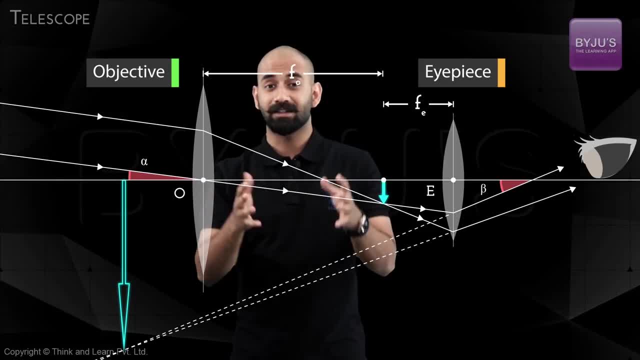 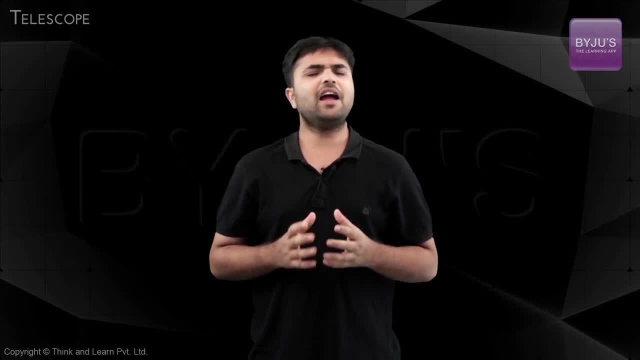 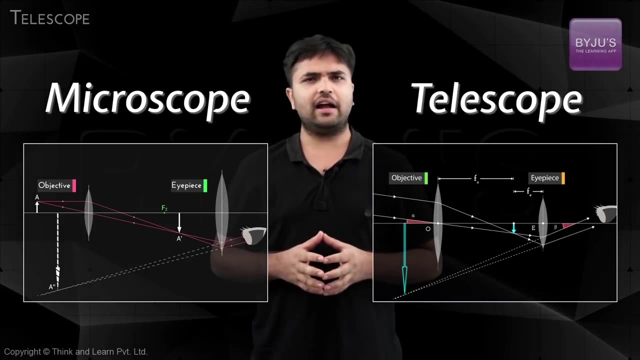 actually it looks like the object is much closer, and that's how telescopes work. hey, Avinash, all beautiful, but I have a doubt. you know, microscopes and telescopes have almost similar working right. they both have two converging lenses and two-step image formation, then magnification. 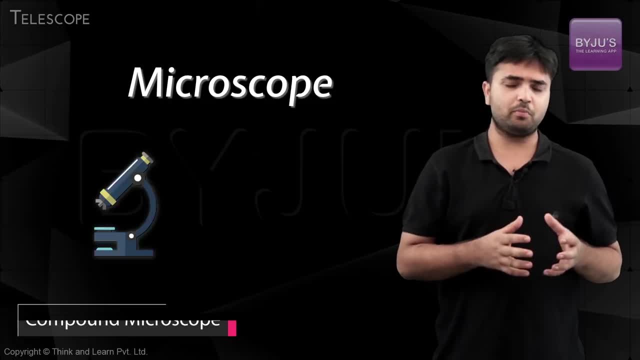 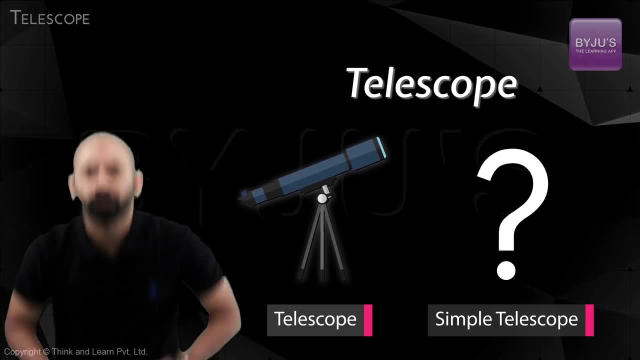 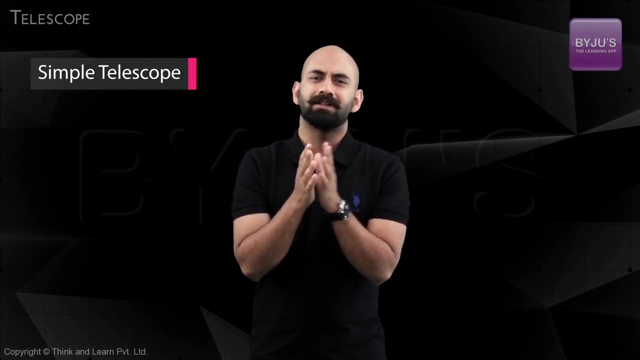 but we had two versions of a microscope: a compound microscope and a simple microscope. I remember why don't we have a simple telescope? okay, so why no simple telescope? let's see. so what do we need for us to achieve what a telescope does with a single convex lens? 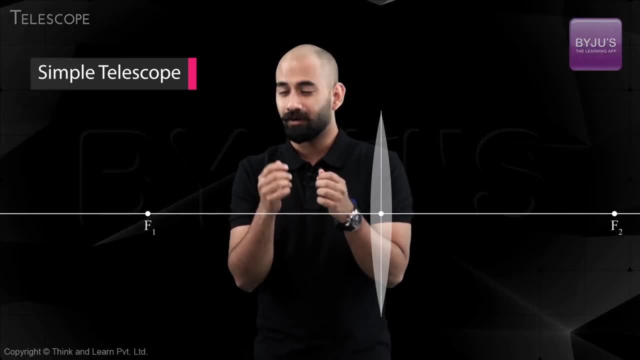 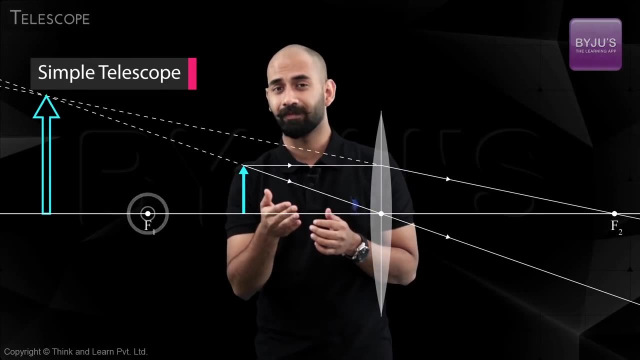 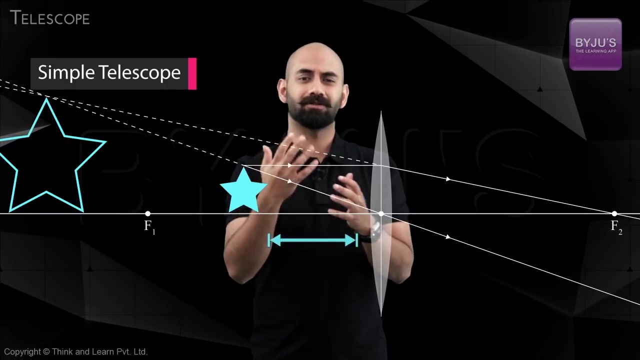 so we need to create a magnified image of a magnified virtual image of the object with a single lens, but to do that, the object has to be within the focal length of the lens, right? so in this case we are dealing with objects that are really far like stars, for example, which are what a few light years.